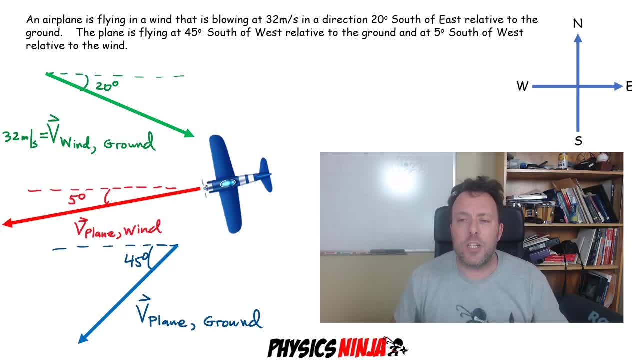 questions based on all of this information here. My questions are: how do you calculate the magnitude, the speed of the plane relative to the ground and also the speed of the plane relative to the wind? What is the length of both of those, the red vector and that blue vector? All right, we're going to set up the vector equations. I'm 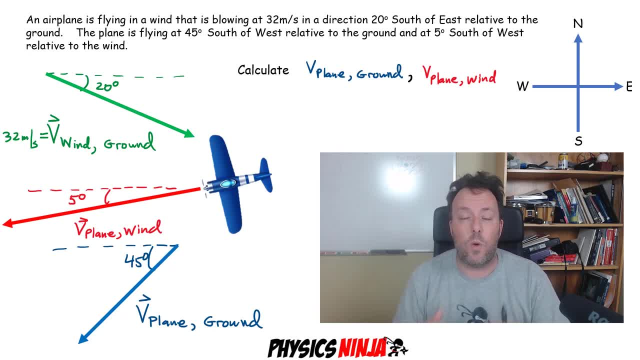 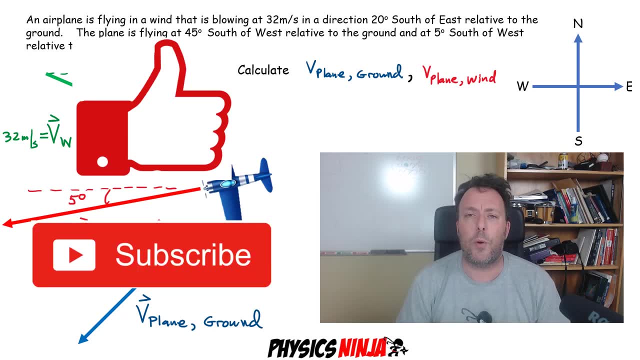 going to set up the vector diagram. We're going to see how we solve for both of these quantities. Like with all my videos, if you like it, give it a thumbs up- Consider subscribing to Physics Ninja. It's the best way to support what I do. All right, let's get started. 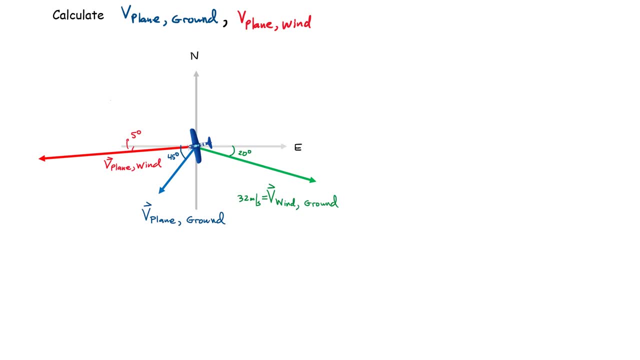 All right, to get this problem started. what we're going to do is I drew the vectors now started all of them, So I'm going to start with the first one. So I'm going to start with the first one, All three of them at the origin. All right? so we've got the green vector. That's the velocity. 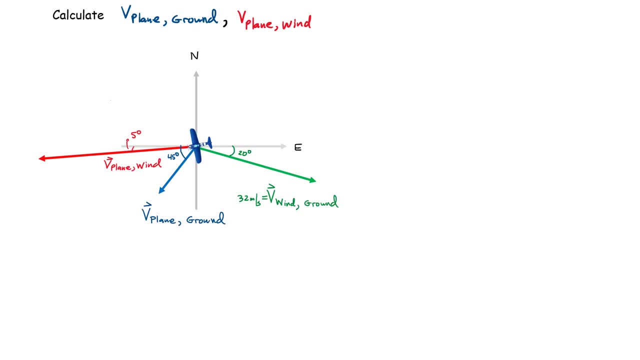 of the wind relative to the ground. This vector, we know its magnitude, which is 32 meters per second, And we also know its direction, which is 20 degrees. What is that? South of east? Now we're told that the plane flies relative to the wind over here. That's the red vector. 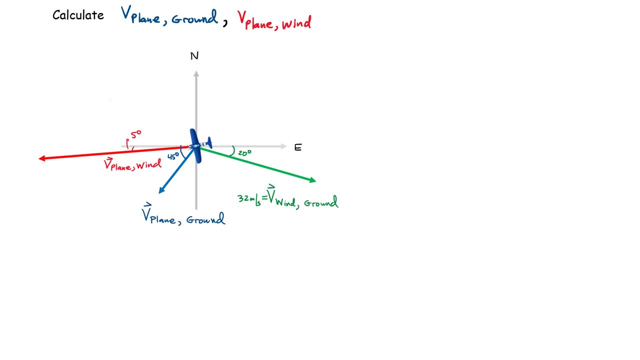 That is at five degrees. We're not told the magnitude of that, but that's one of the questions is: how long is that vector? And the other thing we have is the velocity of the plane relative to the ground. So we're going to start with the green vector, That's the velocity of the 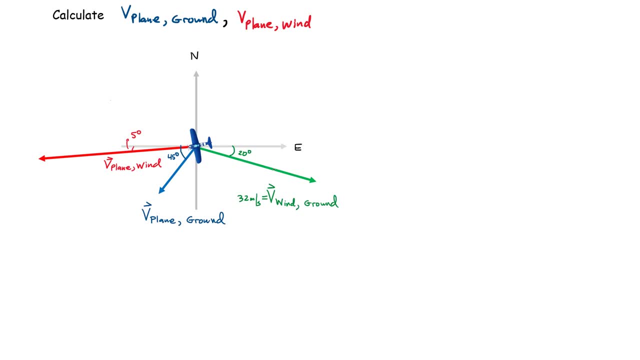 to the ground. Okay, we also know its orientation over here. So, if you think about it, here we have the plane that's flying in this red direction, right relative to the wind, but the wind is pushing it. So at the end we end up in this direction of the blue arrow right here, because 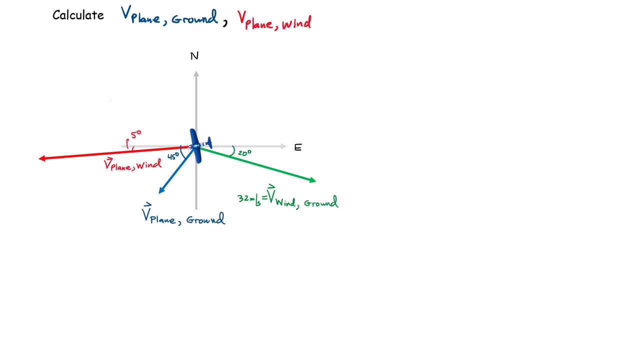 of that strong crosswind over here. So how do we set up a vector equation to link up these three vectors together? Well, this is what it looks like, All right, so I'm going to just write one equation, For example, imagine I wanted to write the velocity of the plane. So I'm going to write: 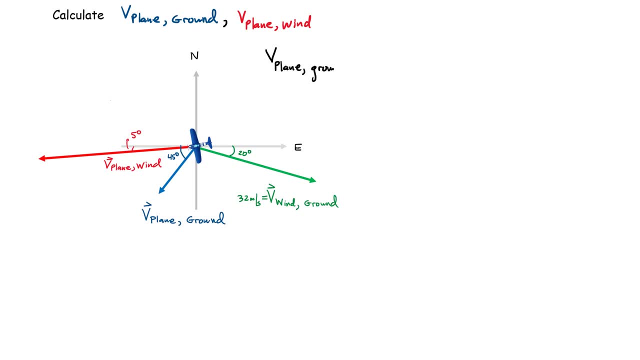 the velocity of the plane relative to the ground. Now, there are really three variables in this problem. right, We've got the plane, we've got the ground and what else? We also have the wind that appears in some of those. So my goal now is going to be to insert over here the wind. 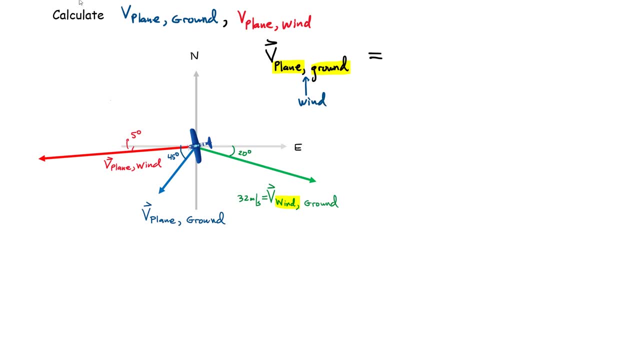 So how do you do that? and write a vector equation. It looks something like this: So you end up writing this as the sum of two vectors. All right, you keep the first term over here. This is the velocity of the plane, And now I insert the wind over here. So I'm going to insert the wind over here. 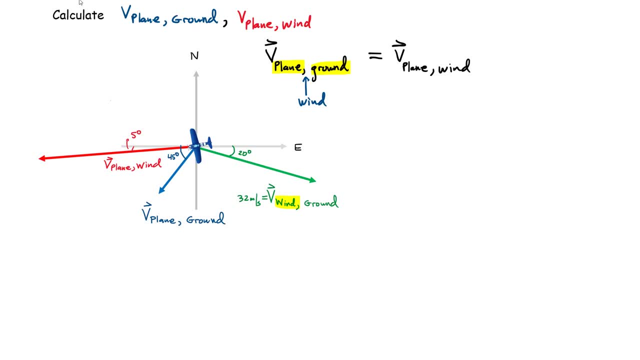 And I introduce my new variable here, which is the wind. Now I want to make this the sum of two vectors. So I said now you have to add a second vector, Now the second vector. well, what you do is whatever variable you've inserted here between the plane and the ground, I also insert it. for. 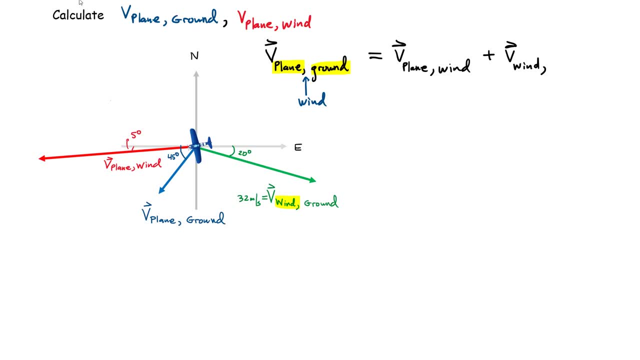 this term. So this is the velocity of the wind relative to something. The last thing we write is simply the ground over here. All right, so this is what the vector equation looks like Now. if you think about it, you can see that the wind is the velocity of the plane. So this is the 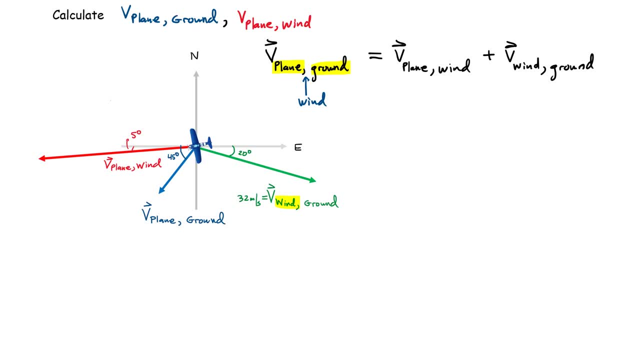 velocity of the plane relative to the ground. Now, if you think about this in terms of the sum of two vectors, well, it says the velocity of the plane relative to the ground, that's the blue vector, equals to the sum of the plane with respect to the wind, that's the red one, and then plus. 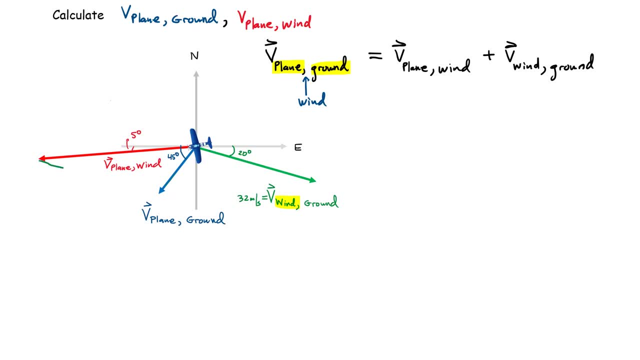 this green one. So if I go over here at the end of the red one and I plot the green one over here, I just move it over. this is the velocity of the wind relative to the ground. So this guy, we actually know its magnitude. This is 32 meters per second. 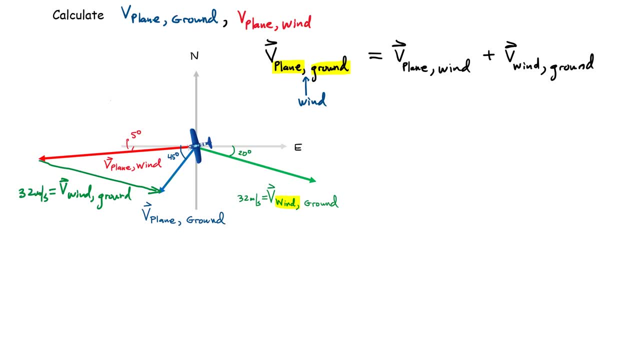 And we know it's 20 degrees south of east. So my goal now is going to be to set up based on this vector equation here. what I could do now is I can break this down. All of these vectors can be broken down into x and y components, And what we're going to do is: 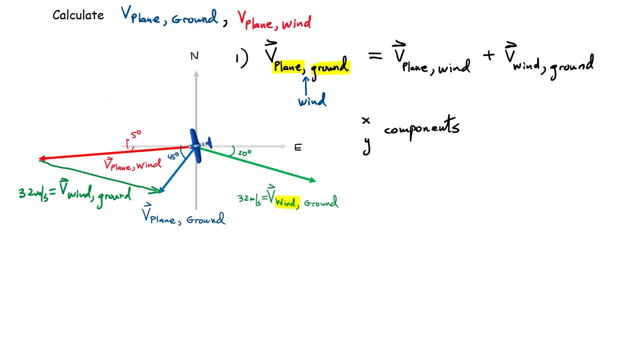 we're going to write two equations based on this vector equations, because this is a two-dimensional problem, So let's keep going and break this vector equation down into two components. All right, so we're looking at the wind relative to the ground and we know it's 20 degrees south of east. 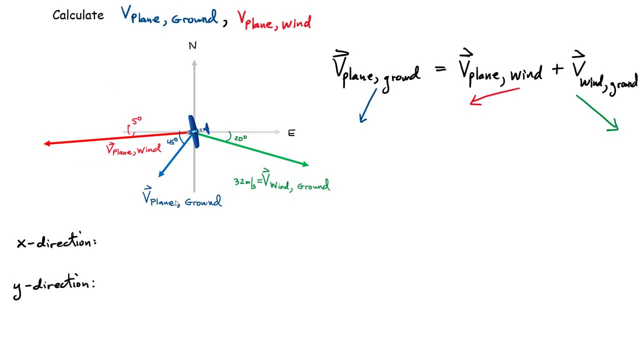 So we're looking at our vector equation. now We're simply writing the vector equation. We can break it down into x direction and y direction. So if we're simply looking at the x component of all of these vectors, then let's take the x component of velocity of the plane. 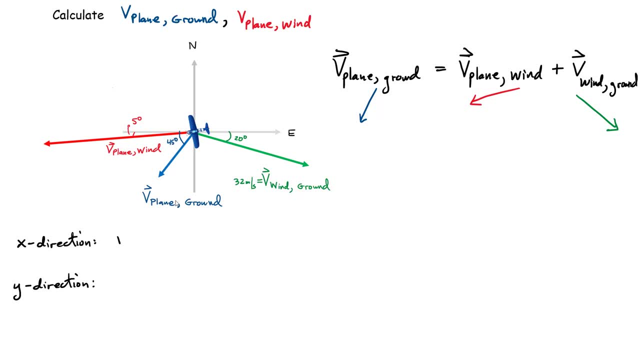 relative to the ground here on the left-hand side. So what you end up getting here is v plane relative to the ground. Now its x component is pointing to the west, So I'm going to put that as a negative answer. And the x component should also have 20 degrees south of east, So I'm going to 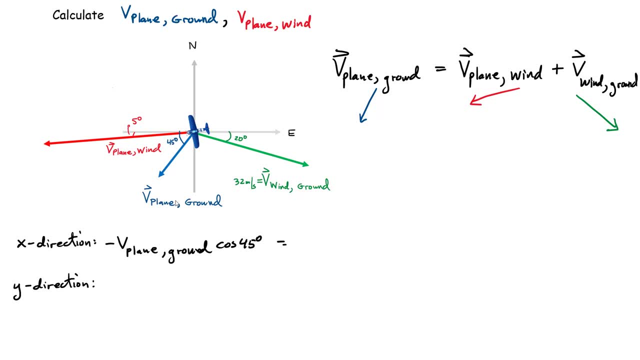 put a cosine of 45 degrees over here, That there must be equal to the sum of the two x components of the red vector and the green vector. For the red vector what you have again is a negative value. This is v plane relative to the wind multiplied by cosine of five degrees. And then 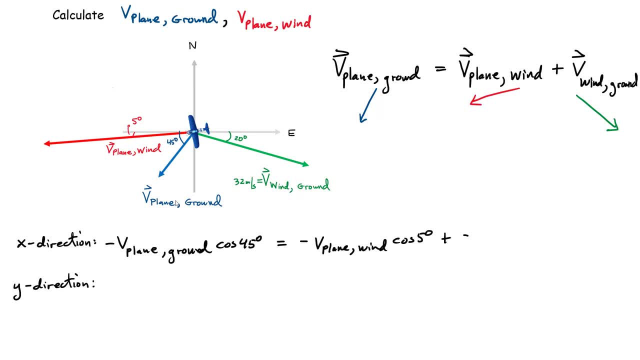 plus again. the x component of the green one is easy. That's simply 32 multiplied by cosine of 20 degrees. All right, So now in the north-south direction, what you end up getting is something that looks like this: You get minus v plane relative to the ground multiplied by sine of 45 degrees, this time. 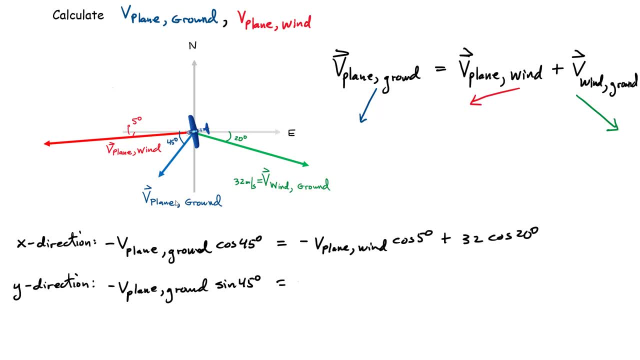 That has to be equal to. again, what is the y component of the red vector? This is minus v plane with respect to the wind, multiplied by sine of five degrees. the negative because it is pointing down that small little red vector component. Now what about the vertical component of the green one? 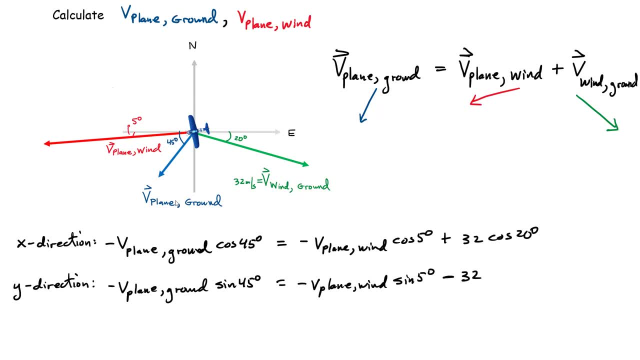 That one's pointing down, So you need to put a negative sign here. That's 32 cosine of 20 this time, Whoa. Let me correct that. We have sine of 20 degrees. Guess what we have now? We have two equations and 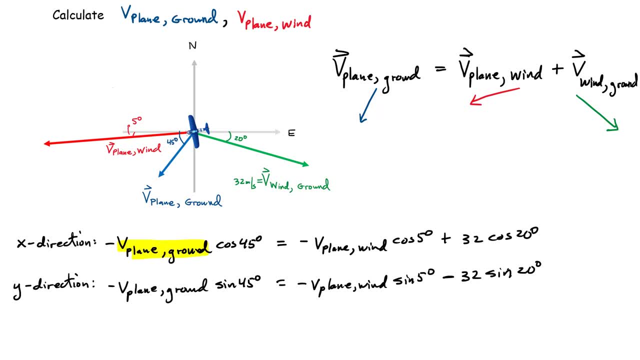 two unknowns. The unknowns are the velocity of the plane that appears over here in both equations, and the velocity of the plane relative to the wind. All right, So that's it. Those are really the two unknowns that I'm trying to solve for in this. 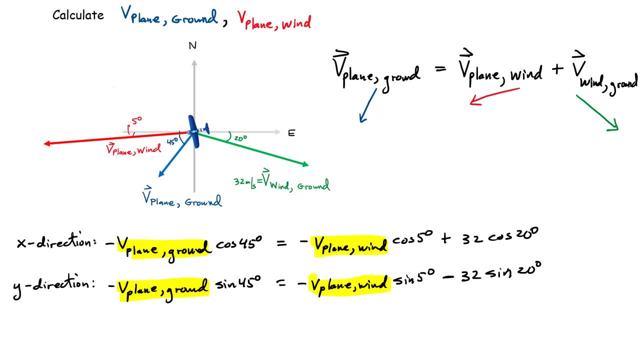 problem. So all you have to do now is simplify and isolate. Now there is a simplification in this case because of the angles that I picked here, And if you know that sine of 45 equals to cosine of 45, that really simplifies this left-hand side of both of those terms. But let's go on the next page now and 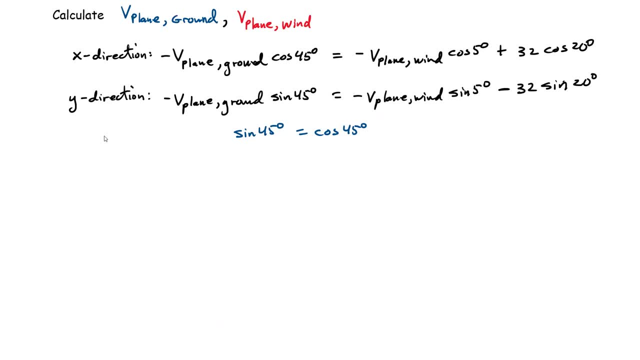 finish off the algebra to solve for both of those unknowns. Okay, So what we're going to do here is I'm going to call this equation A and I'm going to call this equation B, And since the left-hand sides are actually equal to each other, in order to 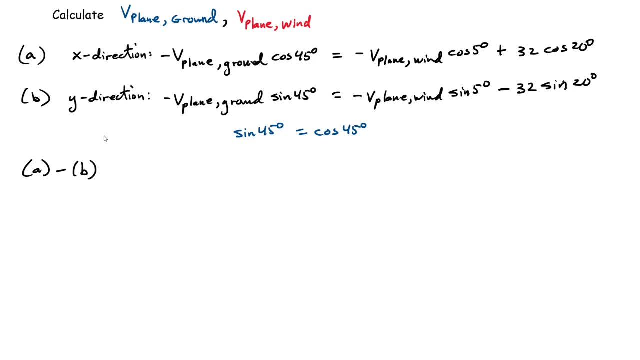 simplify: in order to eliminate one of the variables, all you have to do is simply subtract the two. If I take the difference between A and B, this is what I get. I get zero for this side. If I take the difference now between those, I'm going to get V plane or negative V plane relative to the wind. What else Now I'm? 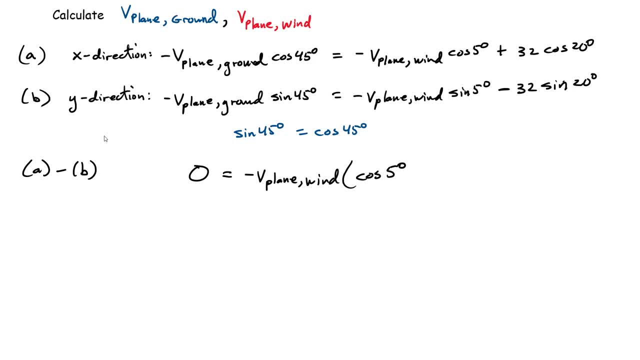 going to open up a bracket. I'm going to have cosine of 20 degrees. I'm going to divide that by the five degrees and then minus sine of five degrees over here on this term. if i'm taking the difference now between both of those terms, what you end up getting here is plus 32 and here you get cosine. 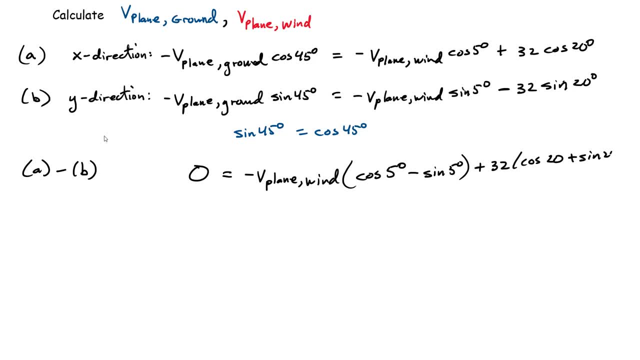 of 20 and plus sine of 20 degrees. all right, the only unknown noun that my problem here is the velocity of the plane relative to the wind. so right away you should be able to write this velocity of the plane relative to the wind. you bring this on the other side. that'll get rid of that negative. 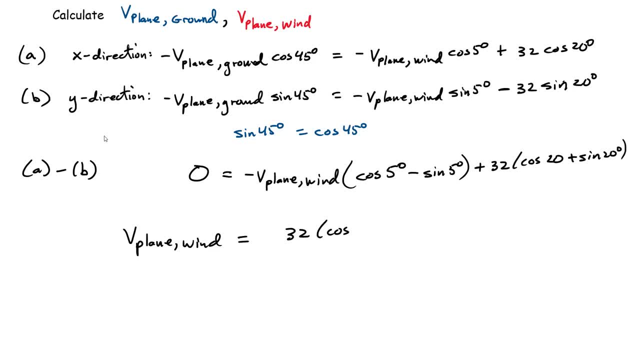 sine. so you're going to be left with 32 cosine of 20 plus sine of 20 degrees. all of this divided by this difference over here, cos of five degrees minus a sine of five degrees. all right, if you put that in the calculator you should get something that is around a 45.1 and that should be measured. 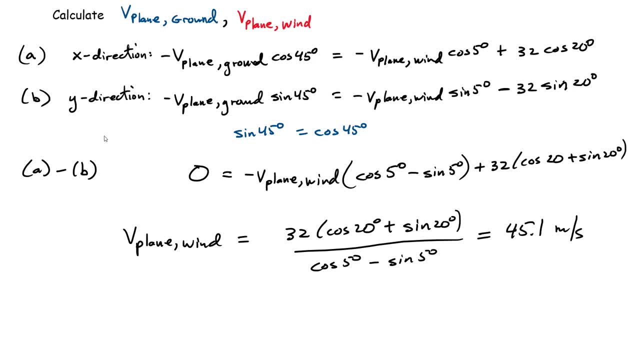 in meters per second. so that is the speed of the plane relative to the wind. that was my red vector on that previous diagram. all right, what's left? we're still left with finding the velocity of the plane relative to the ground. well, we have two equations here that allow us to solve for that: velocity of the plane relative to the ground, or the speed of. 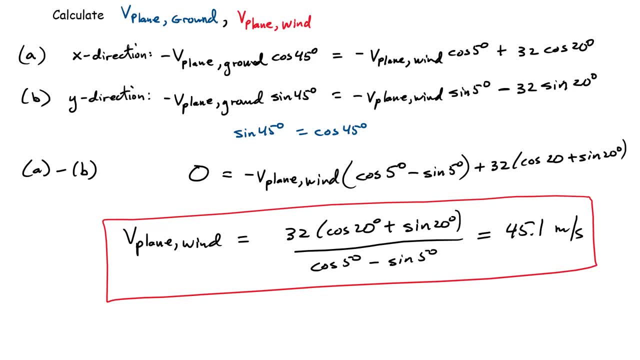 the plane relative to the ground. so all you have to do is simply take one of those expressions and find the answer. all right. so let me take a equation B, for example. right, if you take equation B, notice, you can get rid of those, and what you're left with here is that the velocity of the plane relative to